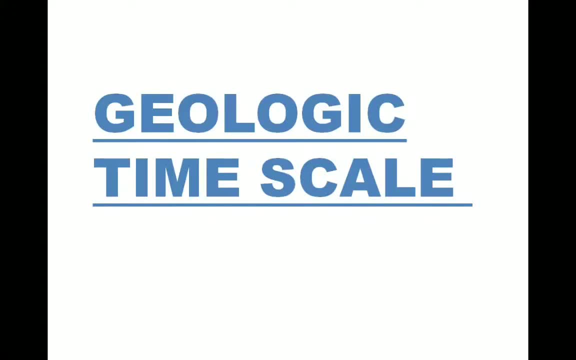 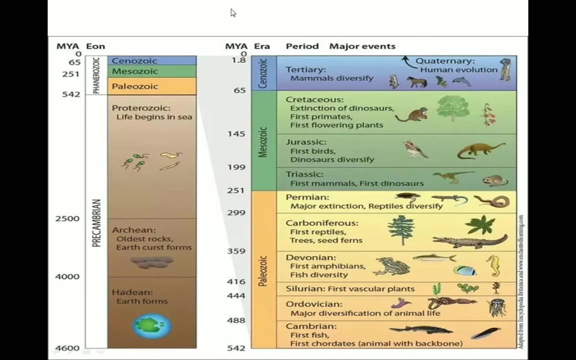 hi guys welcome to my youtube channel geology in this video I will share some information about the geologic timescale but I request if you are new to my channel subscribe to the first channel let's start what is geologic timescale the geologic timescale is a system of chronological dating that relates geological strata to time it is used by geologists paleontologists and other earth scientists to describe the timing and relationships of events that have occurred during Earth's history this is the geologic timescale you can see that eons these are the eons eras periods and major events that have occurred in the Earth's history the largest unit of geologic time is an eon. This is the largest unit and these are the eons. 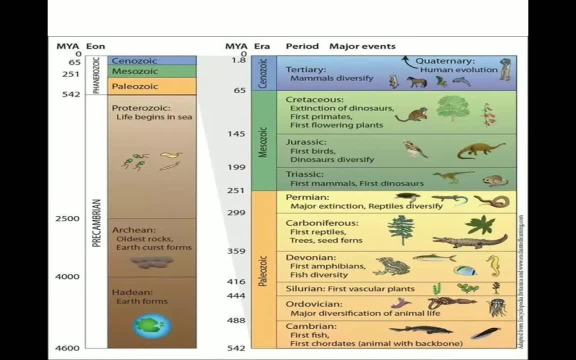 This 4.6 billion year history is divided into four eons, Hedon, Archeon, Proterozoic and Phanerozoic. 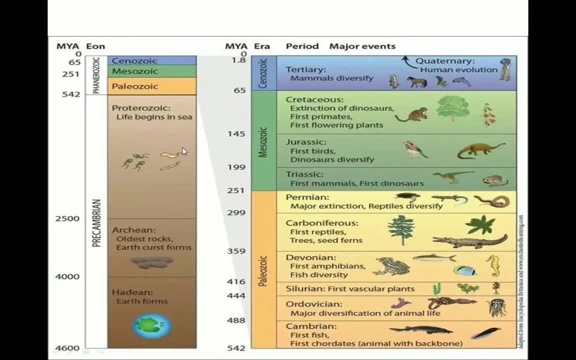 The Hedon, Archeon and Proterozoic eons together are called Pre-Cambrian time. 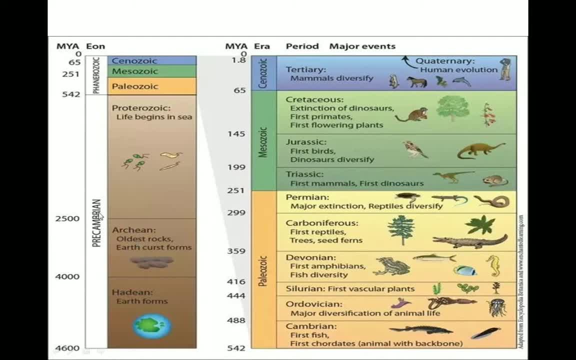 These three eons are called Pre-Cambrian time. 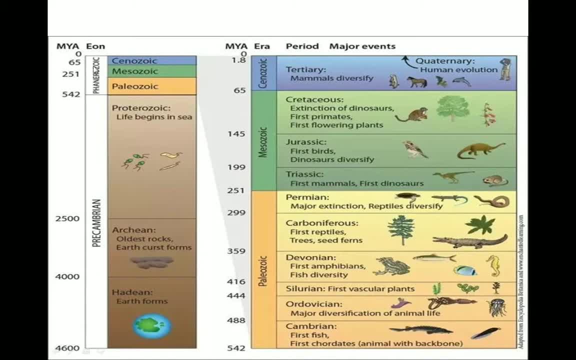 The names of the eras in the Phanerozoic eons are the Cenozoic, Mesozoic and Paleozoic. Cenozoic – recent life, Mesozoic – middle life, Paleozoic – ancient life. The further subdivision of the eras is the Cenozoic, Mesozoic – middle life, Paleozoic – ancient life. 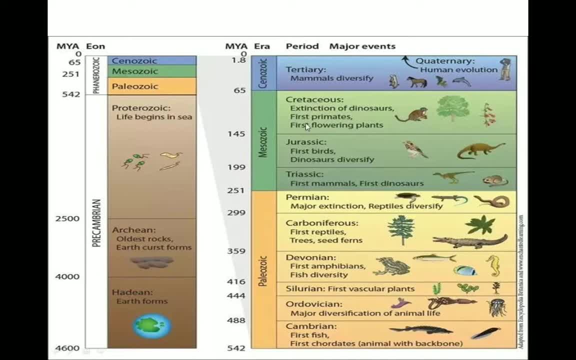 Eros into the twelve periods in the Phanerozoic. 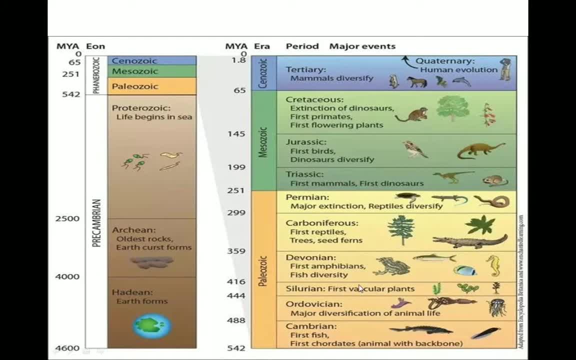 The further subdivision of the eras is based on identifiable but less profound changes in the life forms. Type-2 – Downtown Yeres, 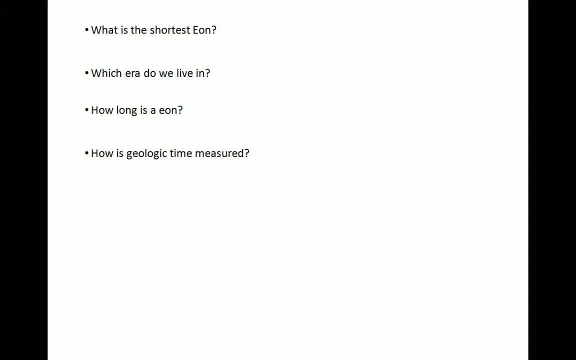 These are some important questions that are often asked, what is the shortest eon, which era do we live in, how long is eon, how is geologic time measure. 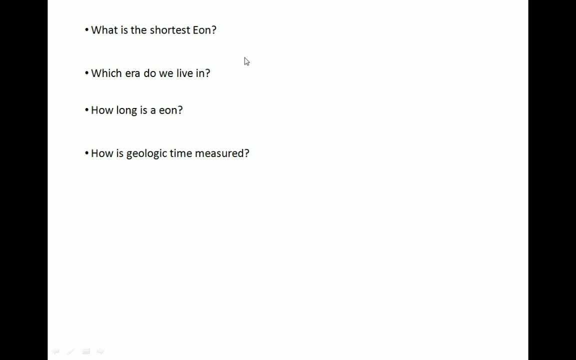 What is the shortest eon, first question is what is the shortest eon. The quaternary spans from 2.58 million years ago to present day and is the shortest geologically 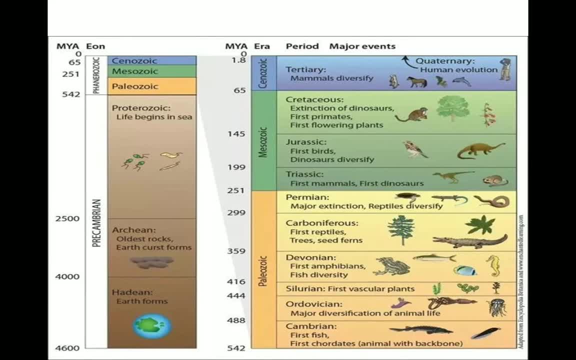 period in the phanerozoic eon. 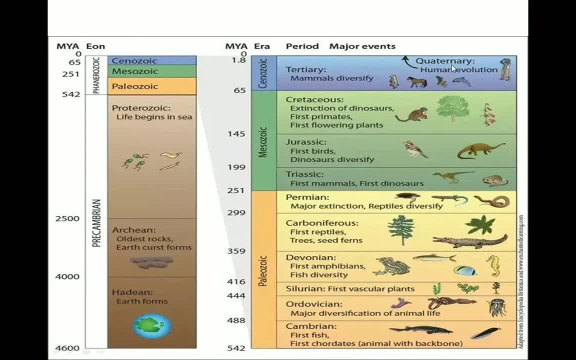 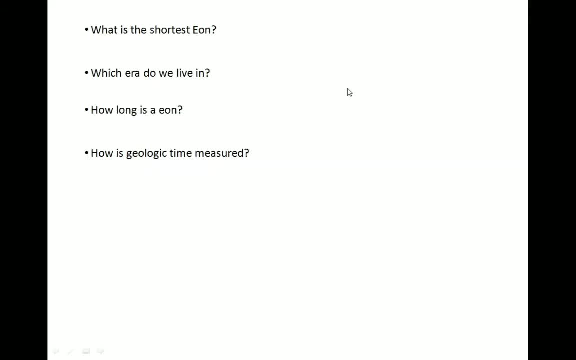 Phanerozoic eon is the quaternary spans of time. This is the shortest eon. Second question is, Which era do we live in? We live in the Polocene, sometimes called recent epoch, contemporary period, Cenozoic 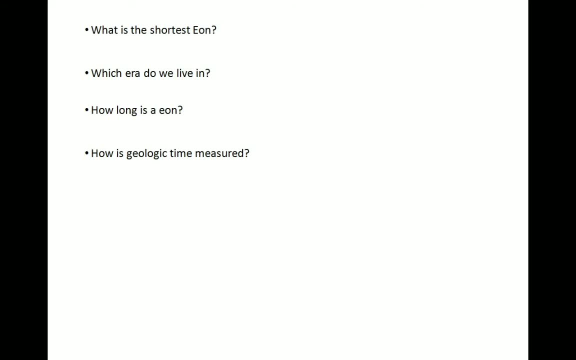 The third question is how long is a eon? About a billion years. 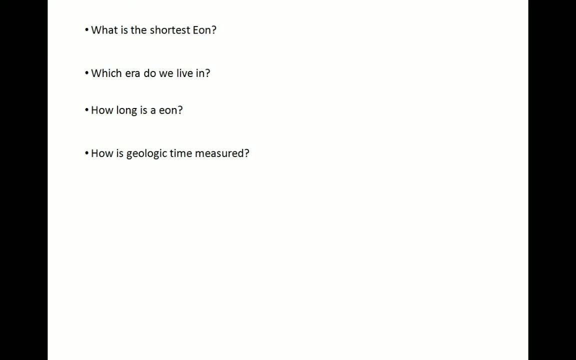 Eon goes back to the Greek eon age and age is not easy to measure and neither is an eon. 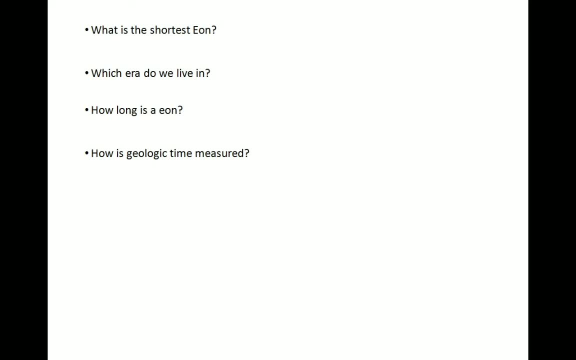 Both are just really long periods of time but in science, an eon is about a billion years. 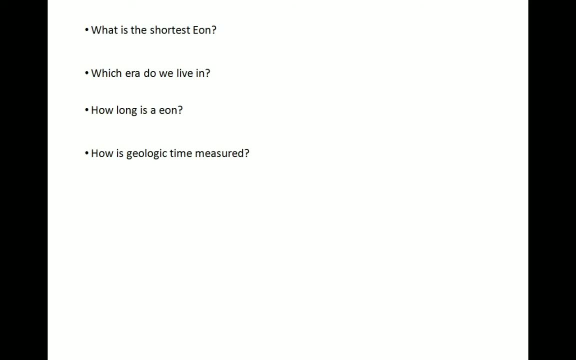 Next, how is geologic time measured? The geologic time scale is a calendar for events in Earth history. It subdivides all time into named units of abstract time called in descending order of 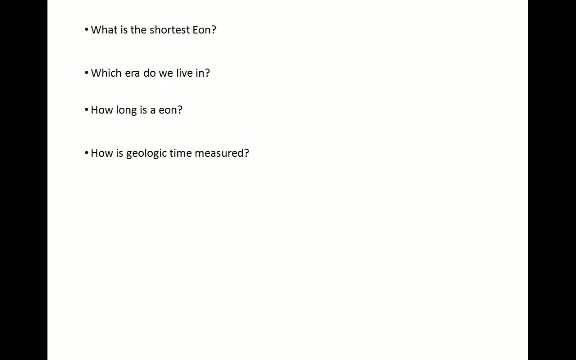 duration. Aeons, eras, etc. Eons, eras, etc. Eons, eras, etc.